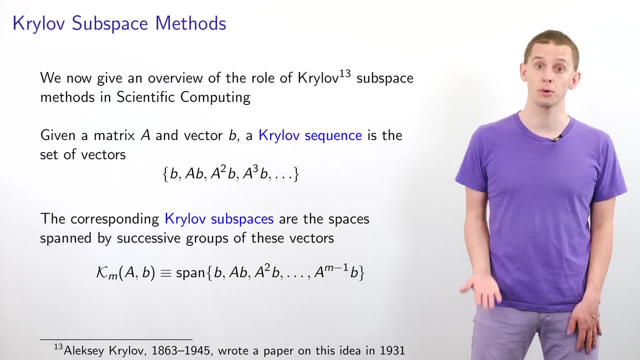 methods family. We now give an overview of the role of Krylov subspace methods in scientific computing And suppose we have a matrix A and a vector B. then we can define a Krylov sequence by repeatedly multiplying B by A, So we can end up with the set of vectors B, AB, A squared B, A cubed B, and so on. 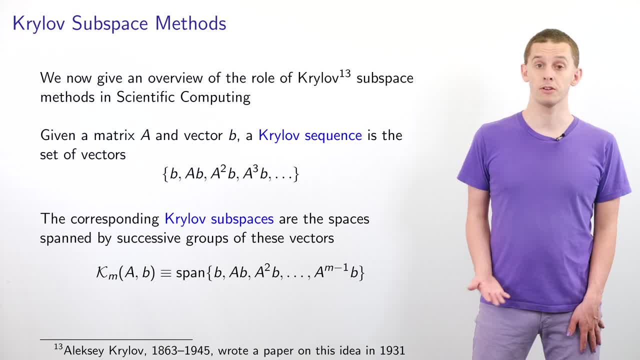 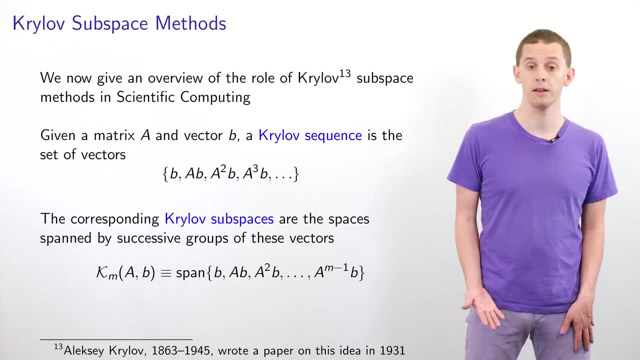 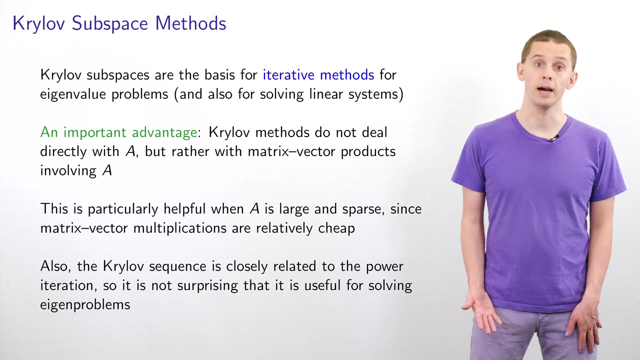 We can define corresponding Krylov subspaces as the spaces spanned by successive groups of these vectors. So KM of AB is defined as the span of B, AB, A squared B up to AM-1B. And these spaces are the basis for iterative methods for eigenvalue problems and they 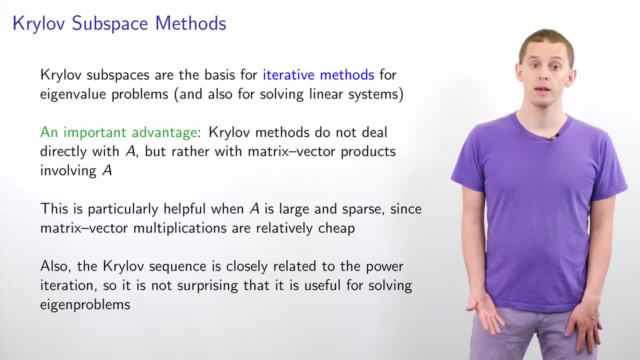 can also be used to solve linear systems. And there's an important advantage in the Krylov method construction in that we don't deal directly with our matrix A, but rather with matrix vector products involving A. So that would be very helpful if we're dealing 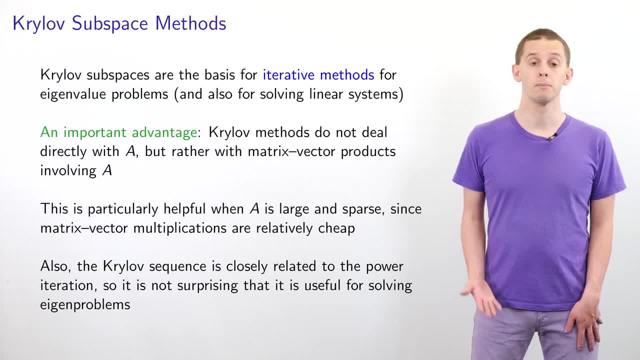 with a matrix A that is large and sparse, because in that case matrix vector multiplication and matrix vector multiplication and matrix vector multiplication can be evaluated relatively cheaply. We can even use Krylov methods in the case when our matrix A might not be available to. 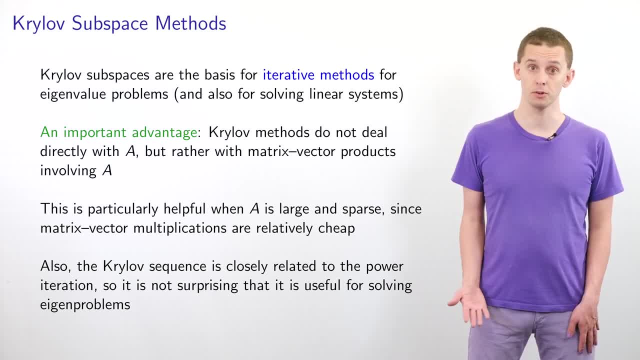 us directly, but could be given to us by some black box function that evaluates the operation and multiplication but doesn't actually give us a way to see the elements of this matrix itself. // still construct a Krylov sequence. in this case, We can also see that a Krylov. 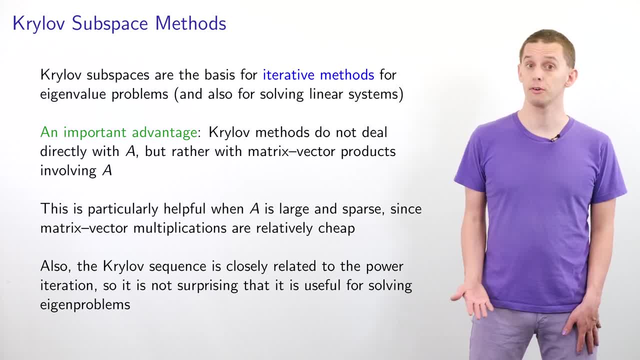 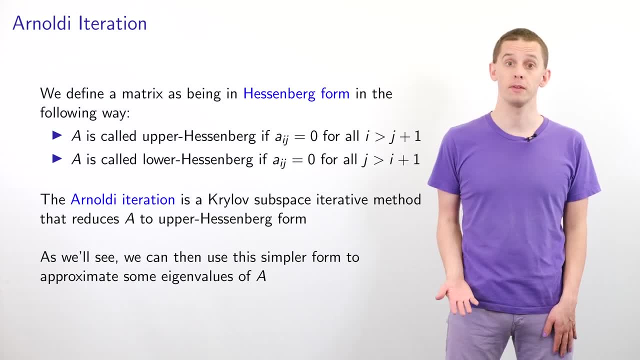 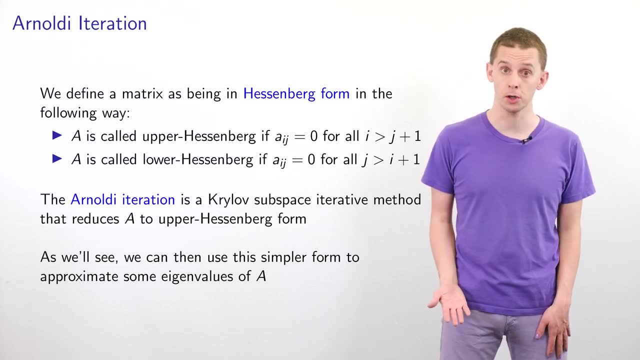 sequence is closely related to a power iteration and therefore it's not surprising that it's going to be useful for solving eigenproblems. The first Krylov method that we'll look at is the Arnoldi iteration, and to begin we'll define a matrix as being in Hessenberg form in the following way. We'll say that: 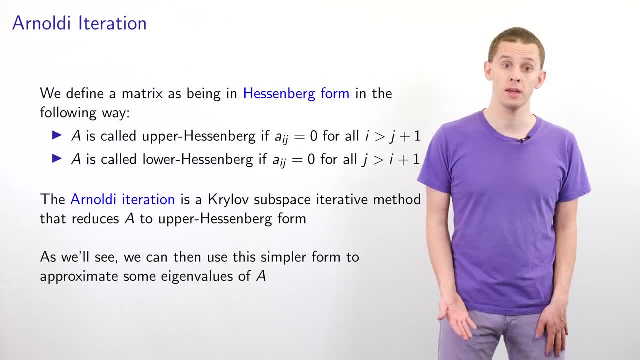 a is called upper Hessenberg if its entries ai, j are equals or zero for all, i greater than j plus 1.. So this is equivalent to an upper triangular matrix, but allowing for terms one below the diagonal, We'll say that a is called. 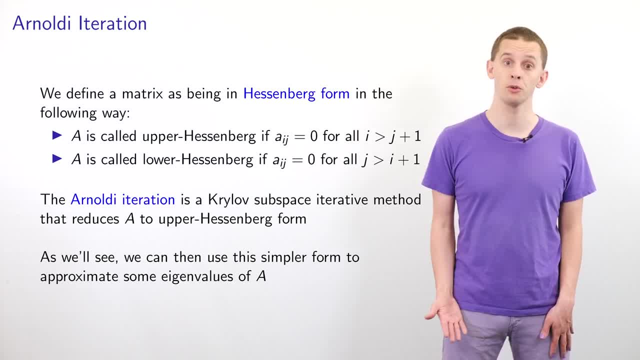 lower Hessenberg if its entries ai, j are equals 0 for all j greater than i plus 1, and this is equivalent to a lower triangular matrix but allowing for entries upper hess telefrag nov one above the diagonal. The Arnoldi iteration is a Krylov subspace iterative method that reduces A. 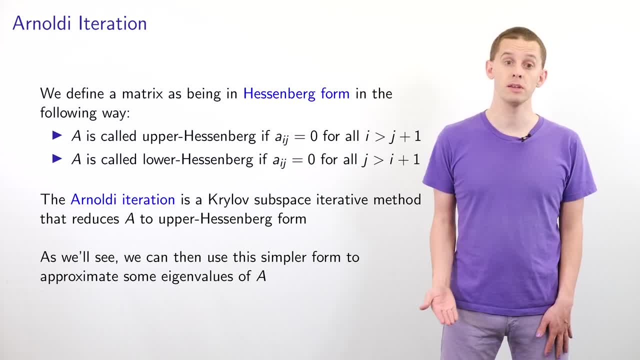 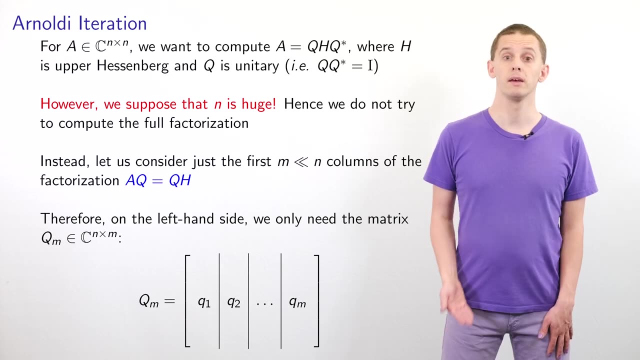 to upper Hessenberg form and, as we'll see, we can use this simpler form to approximate some of the eigenvalues of A. So let's suppose now that A is a complex n by n matrix and we want to compute A equal to q, h q star, where h is upper Hessenberg and q is unitary. So specifically then q- q star. 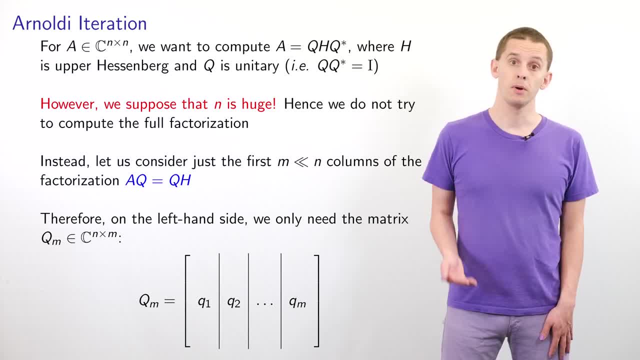 will be equal to the identity. But in this case we're going to assume here that n is huge and therefore we don't want to compute the full factorization. Instead we want to consider some much smaller set m of columns of the factorization. 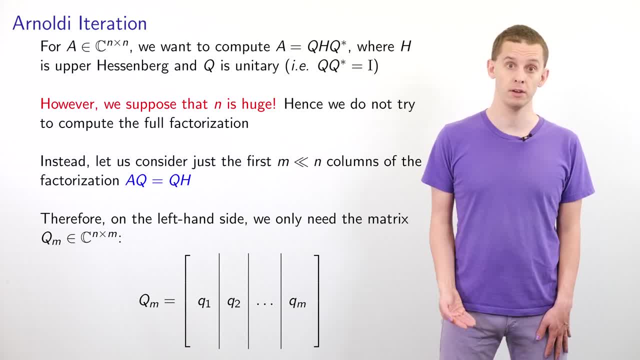 So we'll look here at finding Aq equal q h. So therefore on the left hand side we only need the matrix q m, which is a n by m complex matrix. so we can write here this q m as having columns q 1, q 2 up to q m. on the ritual side we only need the first n and we can use this asStatic. 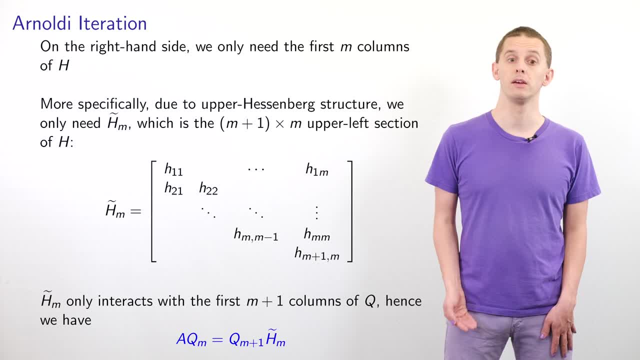 m columns of H and more specifically, due to the upper Hessenberg structure, we only need H tilde m, which is the m plus 1 by m upper left section of H. so H tilde m is shown here. we'll have our upper Hessenberg matrix that is truncated after m plus 1 rows and m columns. 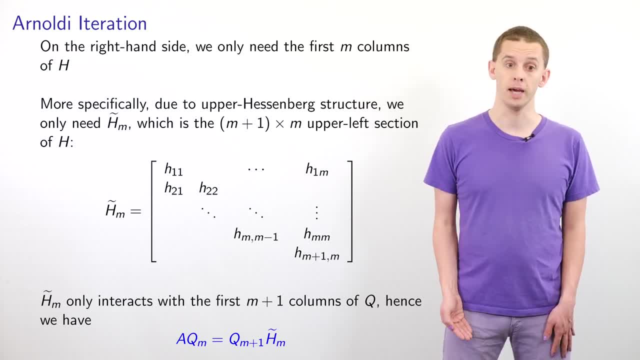 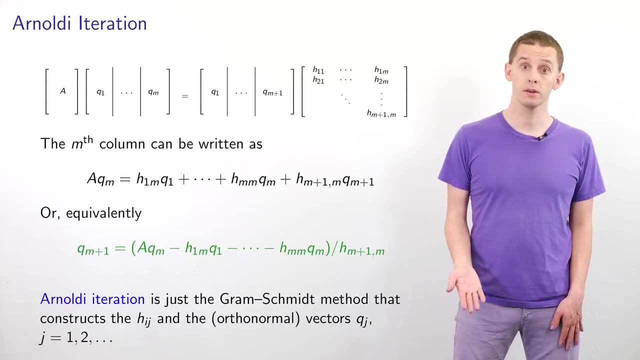 and we see here that H tilde of m only interacts with the first m plus 1 columns of Q, and therefore we have then that A Qm is equal to Q m plus 1 H tilde m. If we look at this diagrammatically. 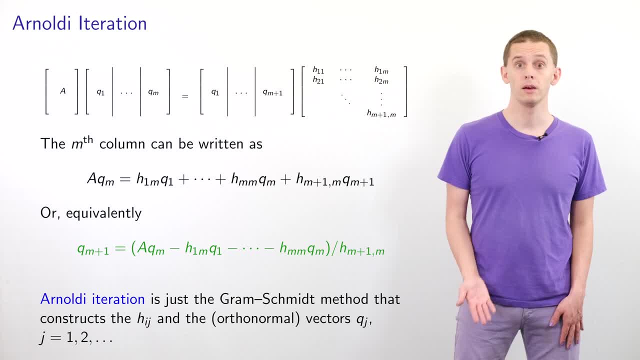 we have that A applied to the first m columns of Q is equal to the first m plus 1 columns of Q applied to H tilde of m. and if we look at the mth column we can see that can be written as A times: Qm is equal to H1m, Q1 plus H2m, Q2 up to Hmm, Qm plus Hm plus 1m, Qm plus 1. 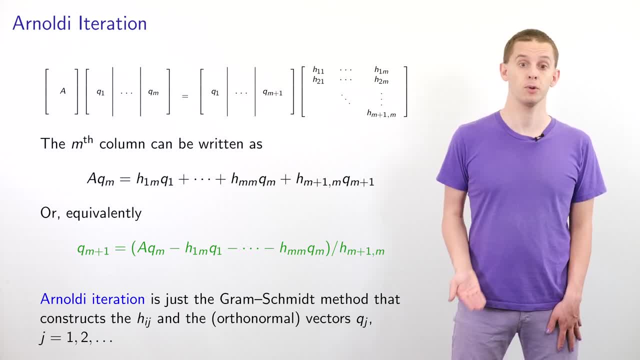 and equivalently we can write that Qm plus 1 is equal to A times Qm minus H1m, Q1 minus H2m, Q2, up to Hmm, Qm divided by Hm plus 1m. and we can see here that the Arnoldi iteration is just the Gram-Schmidt. 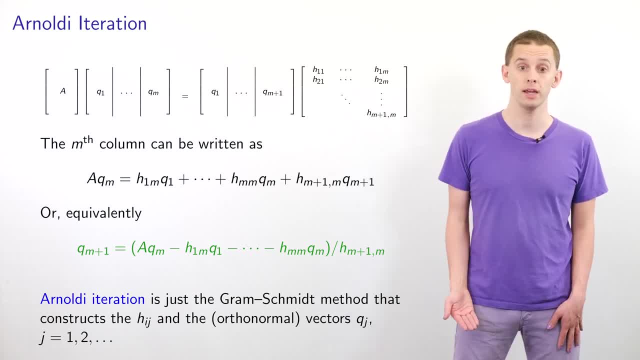 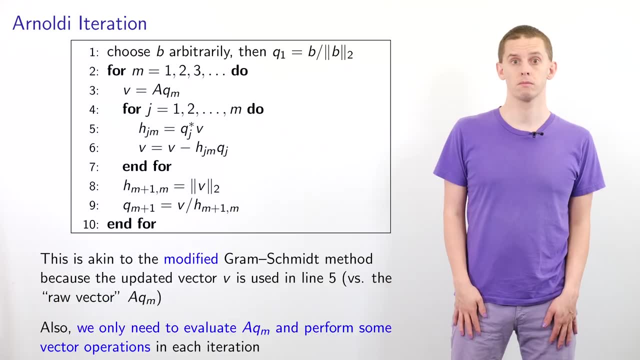 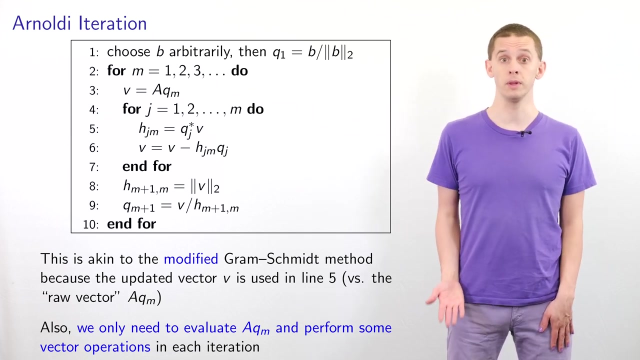 method that constructs the Hij and also the orthonormal vectors Qj. The Arnoldi iteration is therefore very similar to the Gram-Schmidt method that we used to construct the QR factorization, and we can see that in the algorithm we first choose B arbitrarily and we then define Q1 to be the 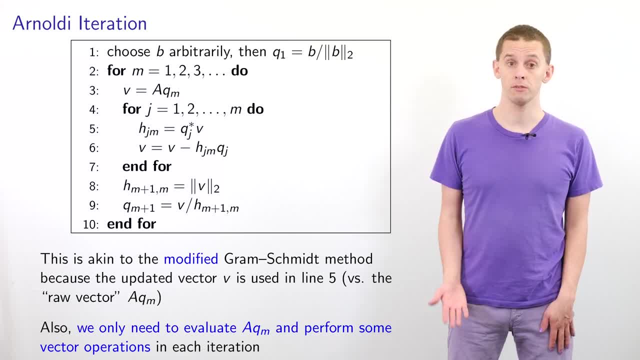 normalized version of B. Then for m equal 1, 2, 3 and so on, we do the following: We first compute V is equal to A times Qm and then we orthogonalize V with respect to all of the previous Q vectors. So for j equal 1 to m, 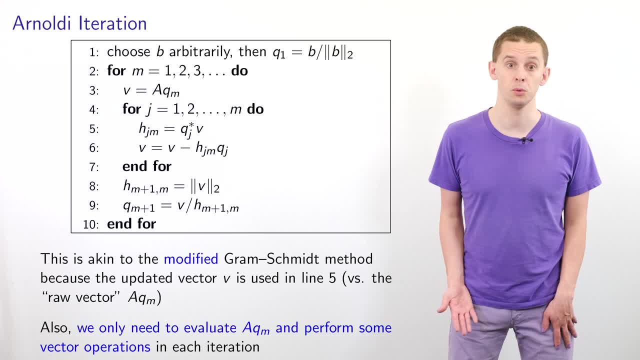 we compute Hjm is equal to Qj star V, and then we update V as V equal V minus HjmQj. After doing this, we compute Hm plus 1m as equal to the norm of V, and we then compute Qm plus 1 as equal to V divided by that norm. 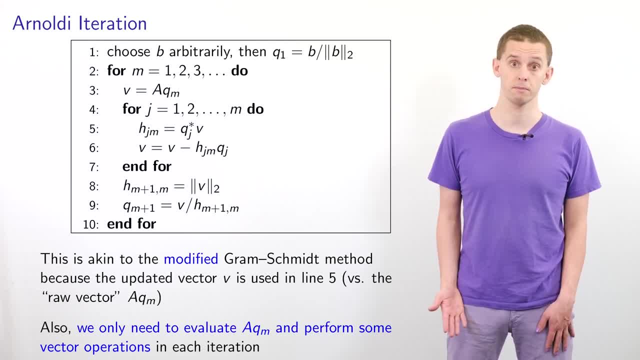 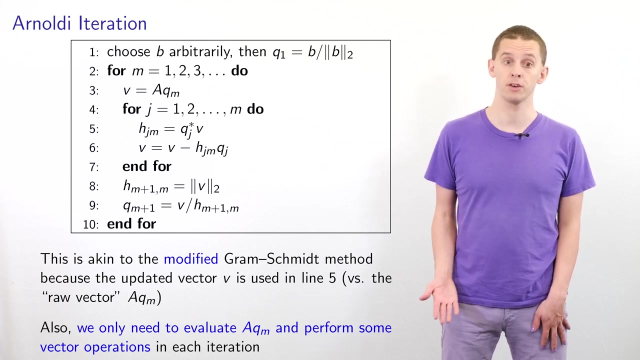 norm to get a orthonormal vector. So this is akin to the modified Gram-Schmidt method, because the updated vector v is used in line five of the algorithm versus the raw vector aqm. In addition, we only need to evaluate aqm and perform some vector. 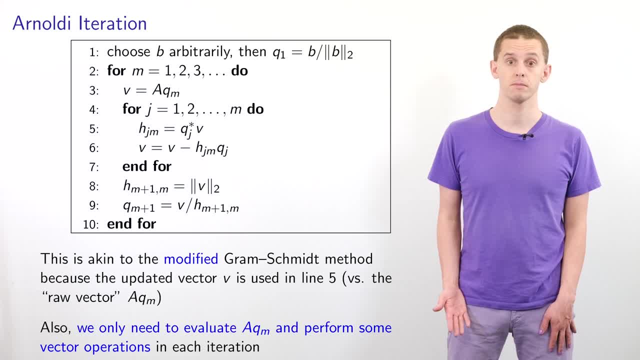 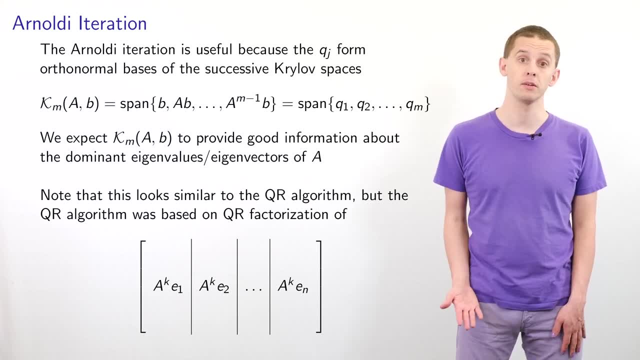 operations in each iteration. The Arnoldi iteration is useful because the qj form orthonormal bases of the successive Krylov spaces. So we see that km of ab is equal to the span of b, ab, a squared b up to a m minus. 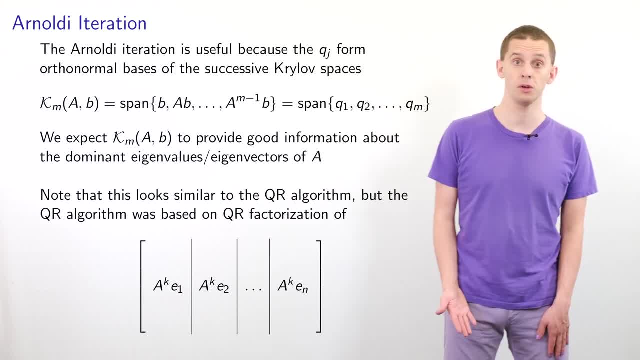 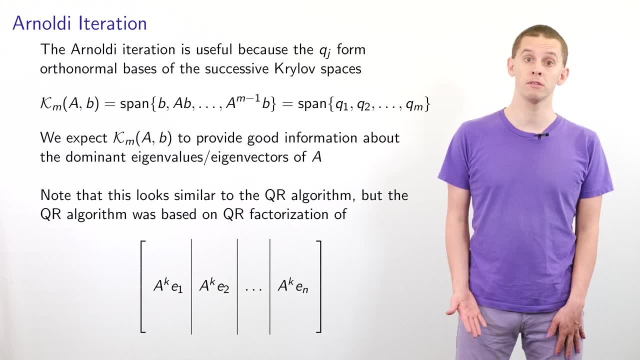 one b, and that will be equal to the span of q1, q2 up to qm, And we expect that km of ab will provide us with good information about the dominant eigenvalues in iqm, And we can note that this looks similar to the QR algorithm, but the QR. 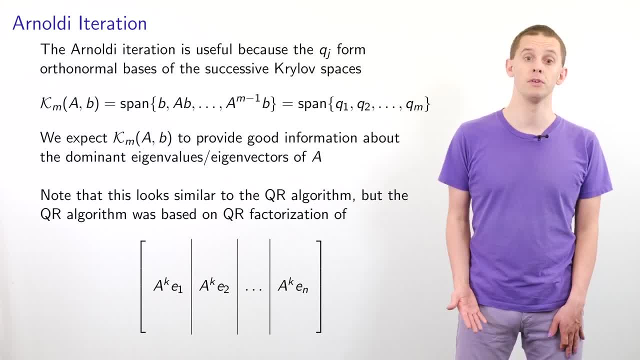 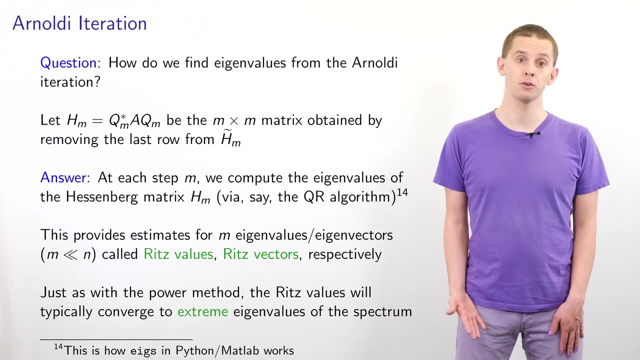 algorithm was based on the QR factorization of the matrix, where we have columns given by a to the ke1, a to the ke2, up to a to the ken. So once we've done the Arnoldi iteration, how do we actually find the eigenvalues? 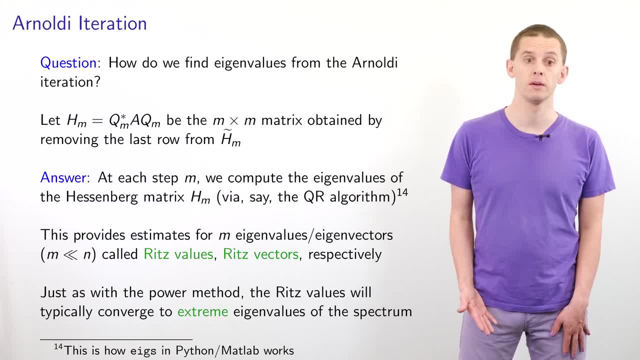 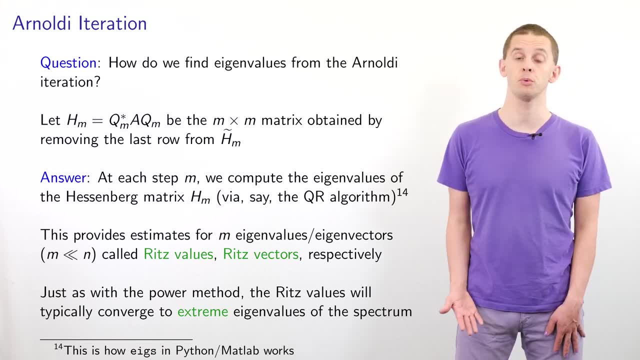 And what we can define here. We can say that the eigenvalue is hm, to be qm, star, aqm, and that will be the m by m matrix obtained. by removing the last row from h tilde m And each step m, we can compute the eigenvalues of the Hessenberg matrix, hm, for example. 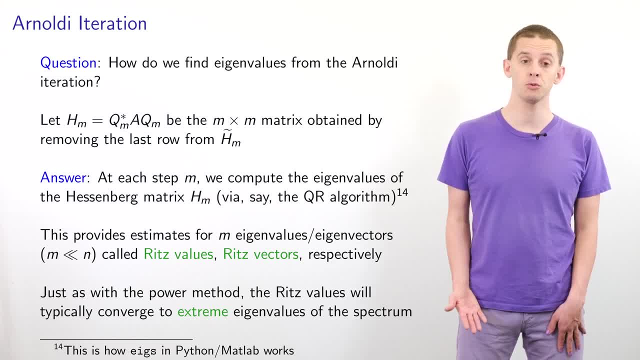 using the QR algorithm and that will provide us with estimates for the eigenvalues and eigenvectors, Specifically the first m, So we can then find the eigenvalues and eigenvectors of our matrix and we refer to these as the Ritz values and Ritz vectors respectively. 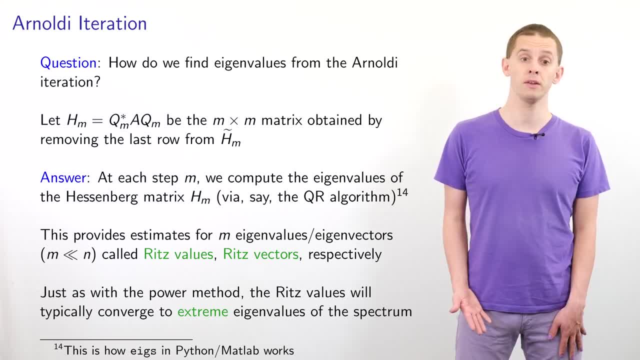 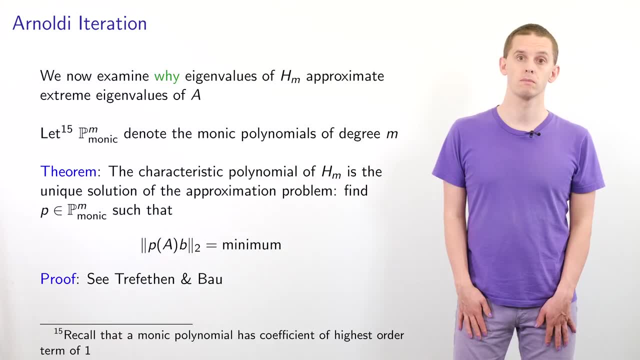 And just as with the power method, we expect that the Ritz values will typically converge to the extreme eigenvalues of the spectrum. We now examine why the eigenvalues of HM approximate the extreme eigenvalues of A, And let PN Monick be the set of Monick. polynomials of degree m. 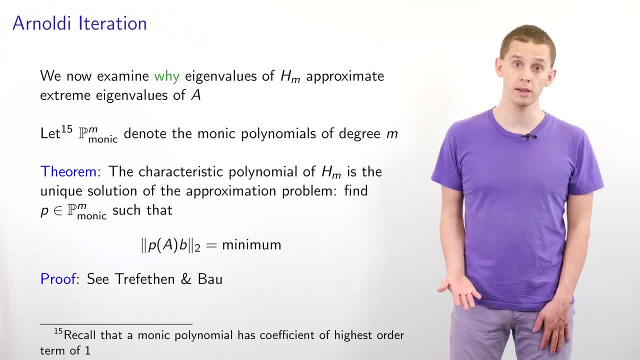 So specifically, this is all polynomials of degree m where the leading coefficient is equal to 1.. So there's a theorem that tells us that the characteristic polynomial of HM is the unique solution of the approximation problem of finding the element P in PN Monick, such that the Euclidean 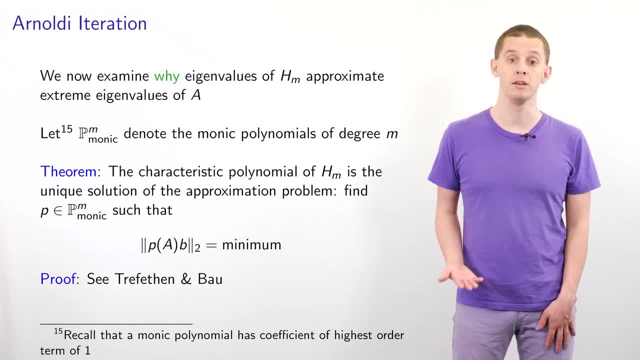 norm of P of A applied to B is minimal. So this is the Euclidean norm of P of A applied to B is minimal. So this is the Euclidean norm of P of A applied to B is minimal, And we're not going to look at the proof here, but the details can be found in the 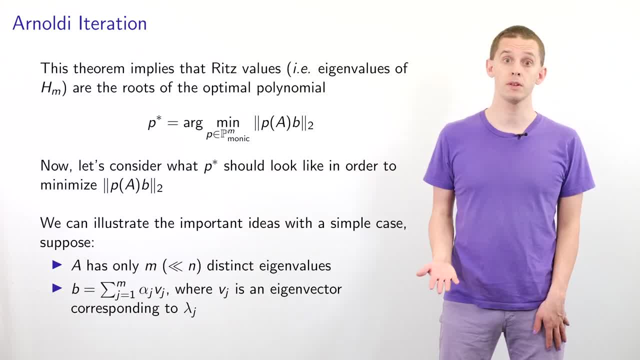 Trefethen and Bao textbook. This theorem implies that the Ritz values, specifically the eigenvalues of HM, are the roots of the optimal polynomial P star. that minimizes the Euclidean norm of P of A applied to B. Now let's consider what P star should look like in order to minimize this Euclidean norm. 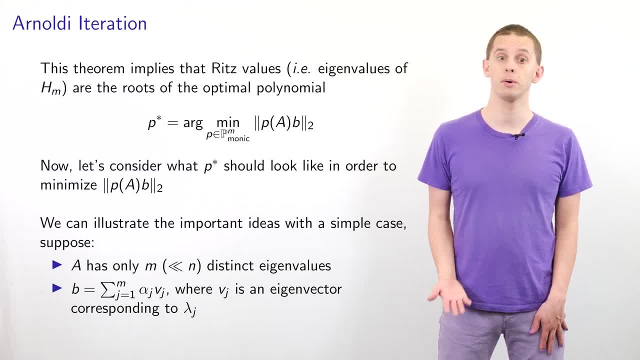 of P, of A applied to B, And we can illustrate the important ideas with a simple case where we suppose that A only has m distinct eigenvalues, much less than the total rank n of the matrix. And let's suppose now that lambda j are those eigenvalues and vj are a set of corresponding. 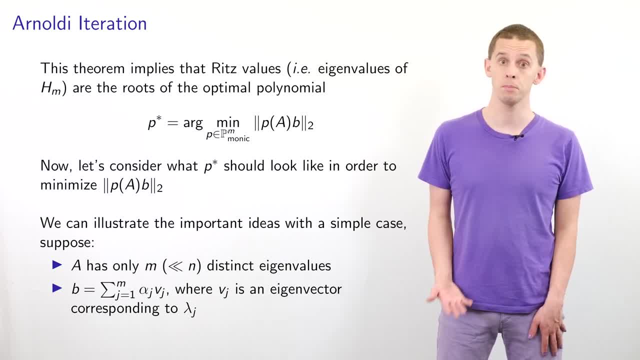 eigenvectors, And let's suppose that our vector B now can be expressed as linear combination of those eigenvectors. So we have then that B is the linear combination of those eigenvectors, And we can write that P is equal to the sum from j to 1 to m of alpha j, vj. 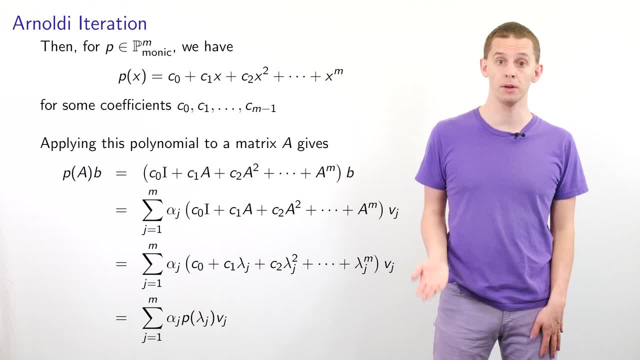 So let P now be a polynomial in PM-monic, And we can write then that P is equal to c0 plus c1x plus c2x, squared up to x to the m, where c0, c1 up to cm minus 1 are the coefficients. 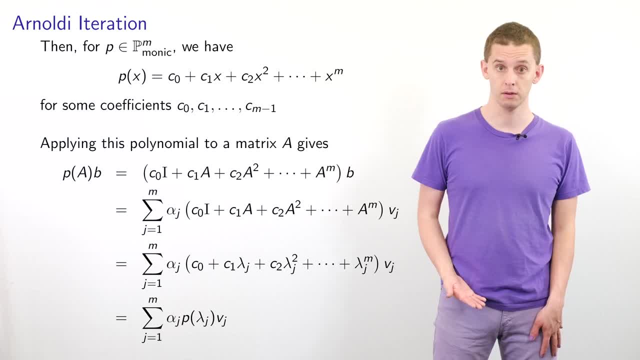 If we apply this polynomial to the matrix A and then multiply it against the vector B, Then we have that P is equal to c0i plus c1a plus c2a, squared up to a, to the m applied to B, And we can now substitute in our expansion for B in terms of the eigenvectors. 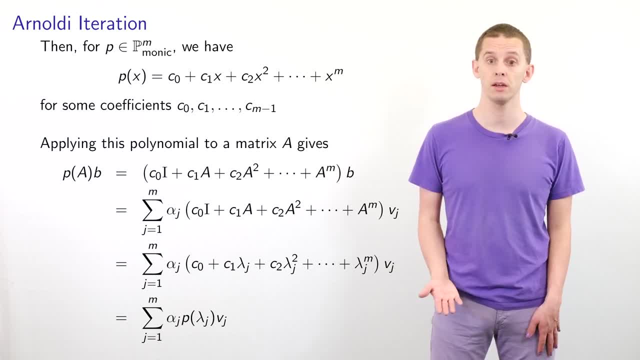 So we have the sum from j to 1 to m of alpha j, c0i plus c1a plus c2a, squared up to a to the m, vj, And that will be equal to the sum from j to 1 to m of alpha j. 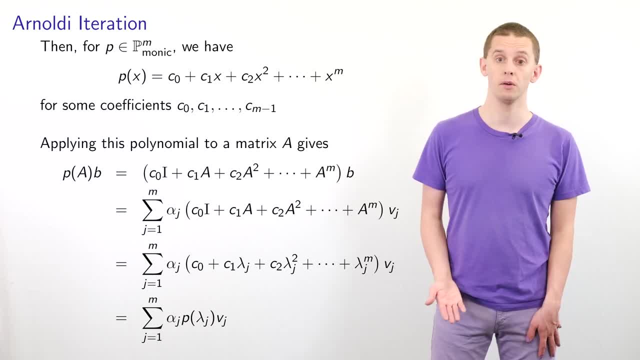 c0 plus c1. lambda j- c0.. c2.. j plus c2. lambda j squared up to lambda j to the m applied to v j, and that will be equal to the sum from j over 1 to m of alpha j times p of lambda j applied to v j. 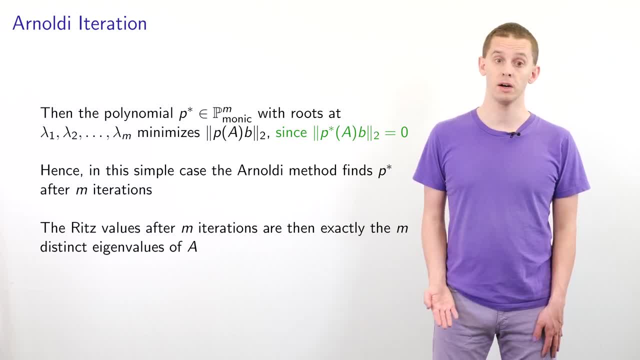 So we see then that the polynomial p star in p m monic that has roots at lambda 1 to lambda n will minimize the Euclidean norm of p of a- b, because in this case p of a- b will actually have zero Euclidean norm. So in this simple case then the Arnoldi method will find the p star after: 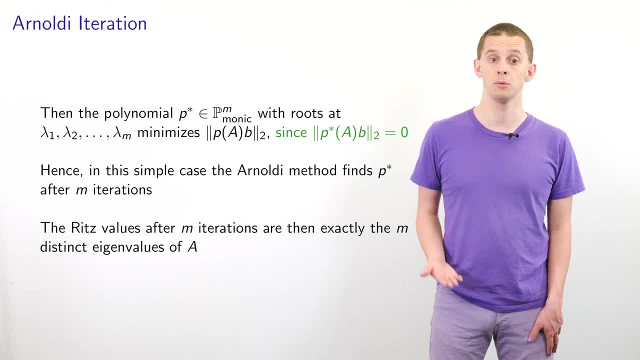 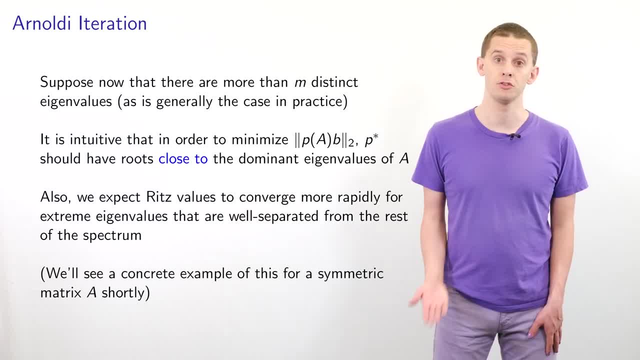 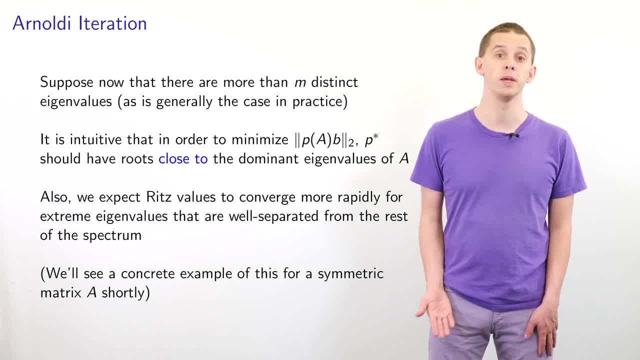 It's intuitive that, in order to minimize the Euclidean norm of p of a, b, p star should have roots that are close to the dominant eigenvalues of a. Also, we expect that the Ritz values will converge more rapidly for extreme eigenvalues that are. 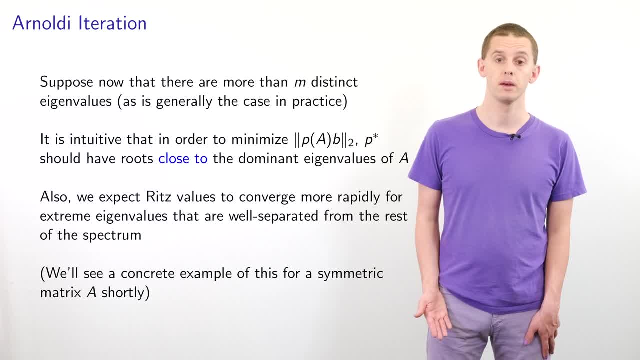 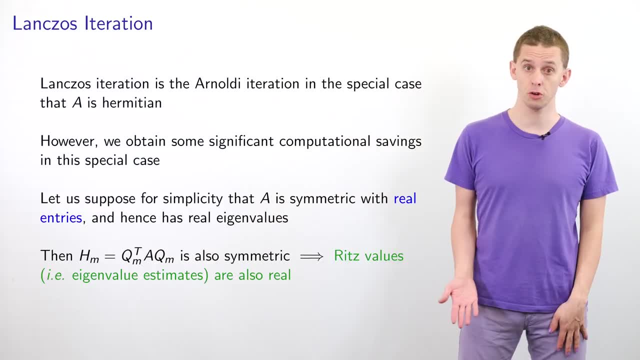 well separated than for the rest of the spectrum, and we'll see a concrete example of this for a symmetric matrix, A. shortly We'll now look at the Lansosch iteration, which is another Krylov method, and a special case of the Arnoldi iteration, when A is hermitian, and we'll see that. 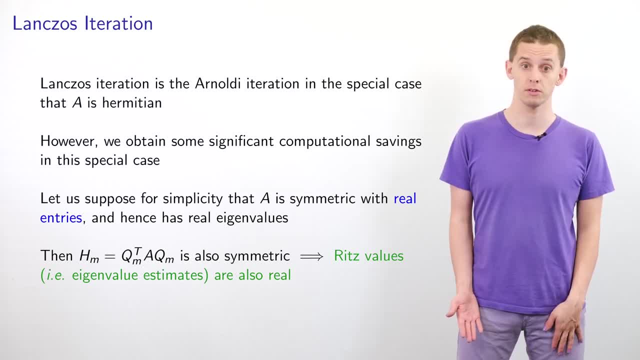 this leads to some significant computational savings. For simplicity, we'll focus on the case where A is symmetric with real entries and therefore it will have real eigenvalues. So HM, which is defined as QM transpose A QM will also be symmetric and therefore the Ritz values. 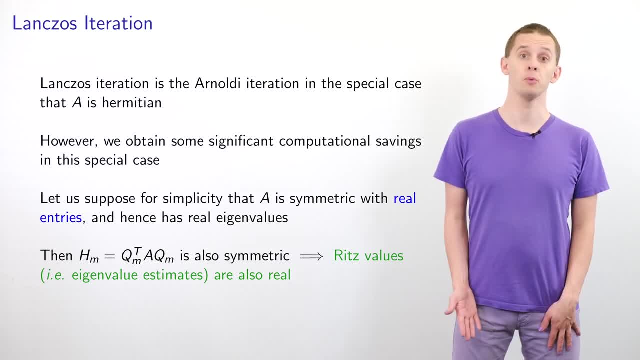 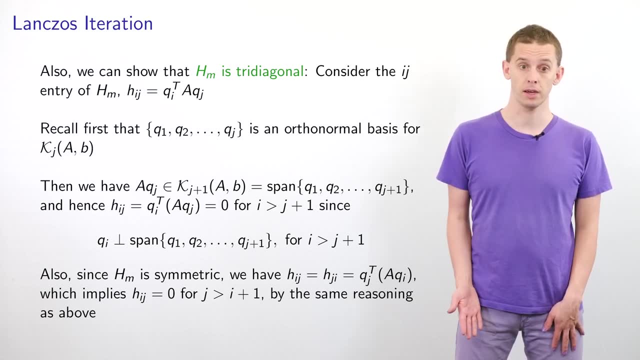 the eigenvalue estimates will be real. We can also show that HM will be tridiagonal in this case, and let's look at the IJ entry of HM. So we have then HIJ will be QI, transpose A QJ, And we recall first that Q1 to QJ is an orthonormal basis for KJ, AB. So therefore we have that A QJ. 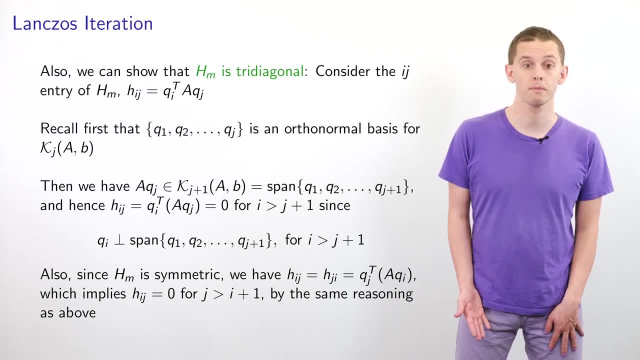 is in KJ plus 1 AB, and that is equal to the span of Q1 to QJ plus 1, and hence HIJ is equal to QI and that will be equal to 0 when I is greater than J plus 1, since we know that QI is perpendicular. 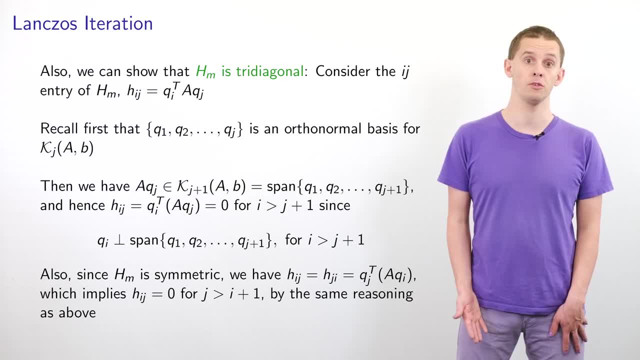 to the span of the Q1 to QJ plus 1, for I greater than J plus 1.. In addition, since HM is symmetric, we know that HIJ is equal to HJI, which is equal to QJ. transpose A QI, which implies then that HIJ. 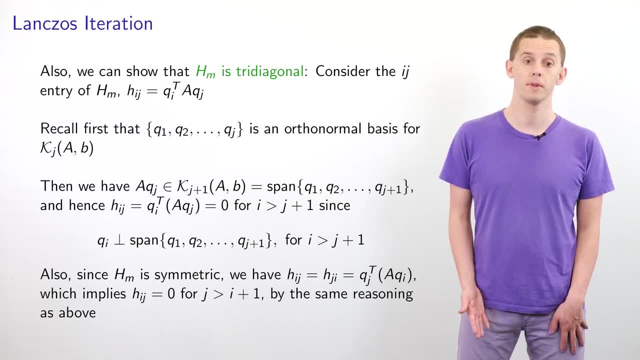 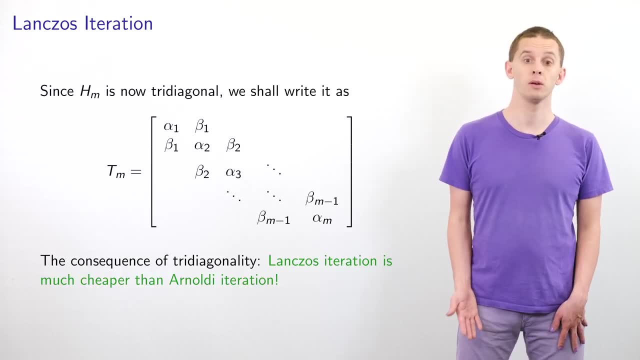 is equal to 0 for J greater than I plus 1, by the same reasoning above. So since HM is tridiagonal, we can write it as TM, where we have terms alpha 1, alpha 2, alpha m on the diagonal and then terms beta 1, beta 2, beta m minus 1 on the sub and super diagonals. So a consequence of the tridiagonality. 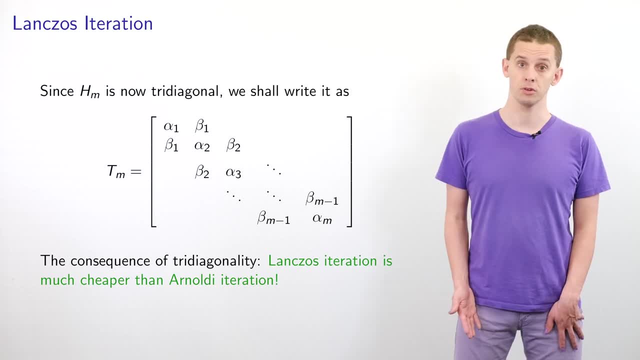 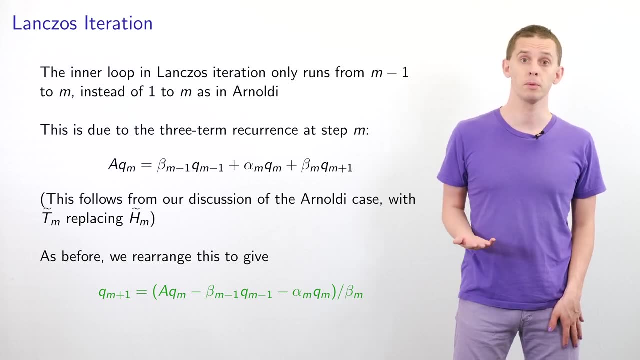 is that the Lansos iteration is much cheaper than the Arnoldi iteration to implement. If we recall the Arnoldi iteration, when we were computing QM plus 1, we had to orthogonalize it with respect to all of the previous Q1 to QM. Here, because of the special tridiagonal structure, we only need to. 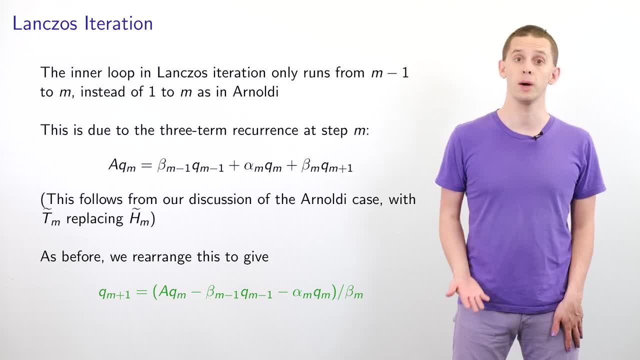 consider orthogonalization with respect to QM minus 1 and QM and we have a three-term recurrence relation. at step m We have that A times QM is equal to beta m minus 1, QM minus 1 plus alpha m. QM plus beta m. QM plus 1, and this follows from the same discussion as the Arnoldi. 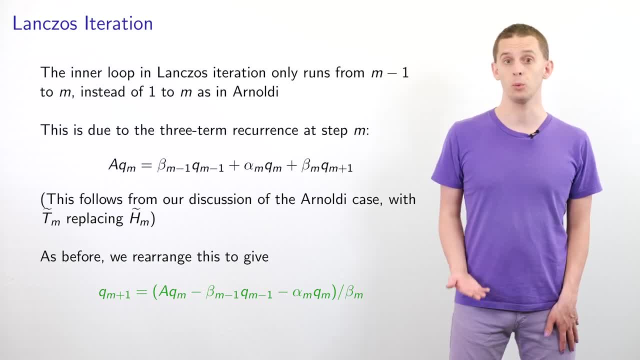 case, but here we've replaced H tilde m with our tridiagonal matrix T tilde m. As before. we can rearrange this to give that QM plus 1 is equal to T tilde m plus 1 and QM plus 1 is equal to T tilde m. 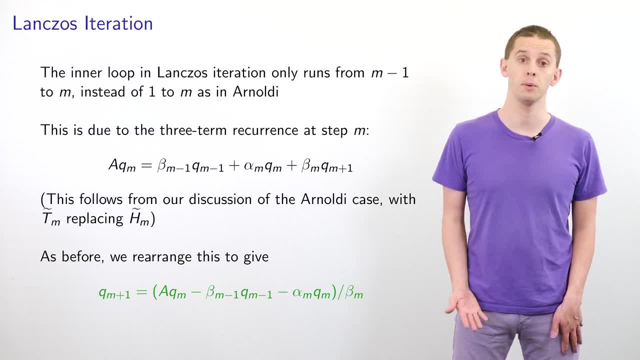 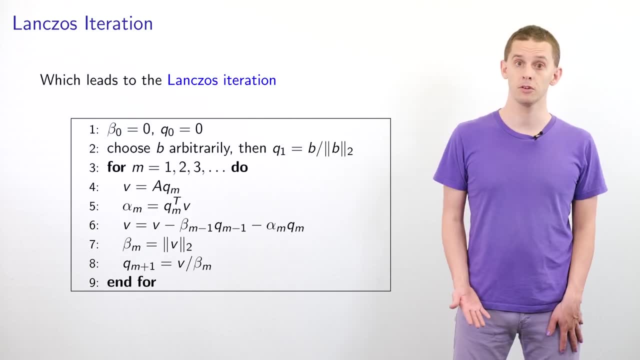 plus 1 is equal to A times QM minus beta m minus 1. QM minus 1 minus alpha m. QM divided by beta m. and that leads us to the Lansos iteration. We first set beta 0 equal to 0 and Q0 equal to 0.. These are: 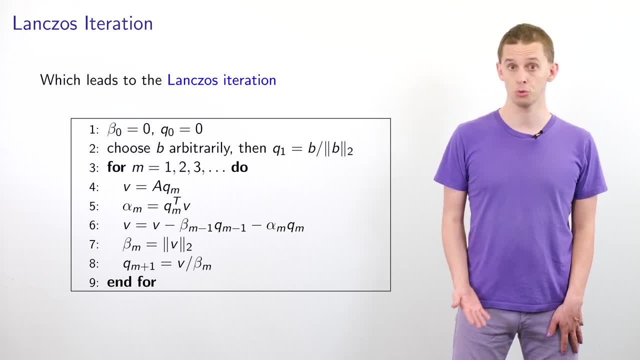 actually outside of our usual matrix. The betas are numbered from 1, but we make these definitions just to handle a missing term in the very first iteration through the loop. So we choose B arbitrarily and we then set Q1 to be the normalized version of B and we then consider m equal 1, 2 and 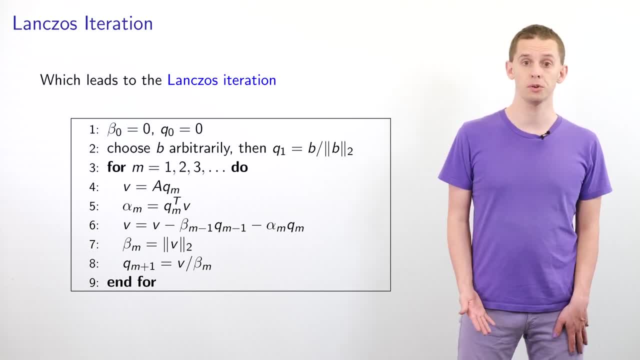 so on. We first calculate V is equal to A times QM. We then evaluate alpha m as QM transpose V. we then compute V is equal to V minus beta m, minus 1, QM, minus 1 minus alpha m, QM and when m equal. 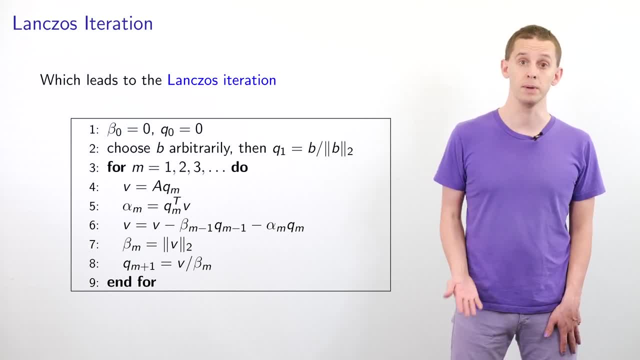 to 1. because of those definitions we will have the. the beta term vanishes here. We then compute: beta m is equal to the Euclidean norm of V, and then we set: QM plus 1 is equal to V divided by beta m. We'll now look at the Euclidean norm of QM plus 1.. We'll look at the Euclidean norm of QM. 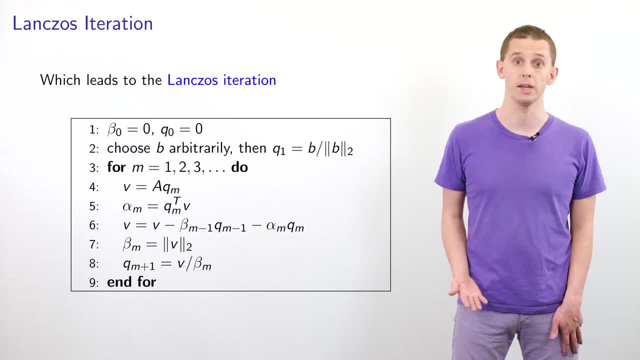 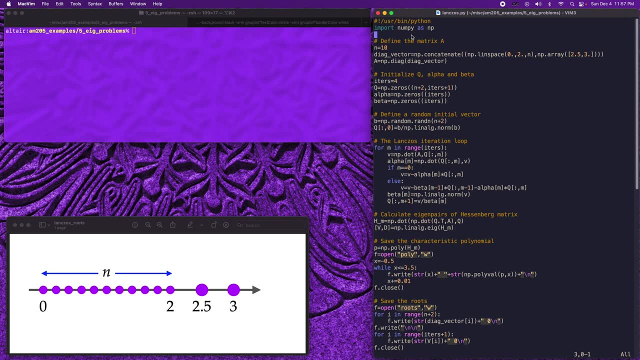 a Python example of the Lansosh iteration in action. Let's now look at the program Lansoshpy. that demonstrates the Lansosh algorithm for finding the eigenvalues of a symmetric matrix, and we're going to test the algorithm on a matrix that has a set of eigenvalues shown in the bottom. 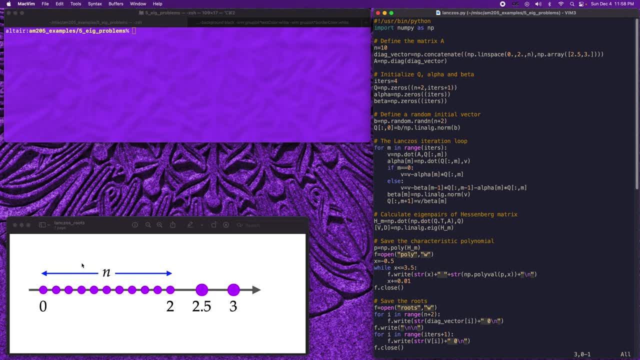 left diagram. We'll make use of n eigenvalues that are linearly spaced between 0 and 2, and then we'll also add in two isolated eigenvalues at 2.5 and 3, and we know that the Lansosh algorithm is particularly good at finding eigenvalues that are isolated in the spectrum, and this is a useful 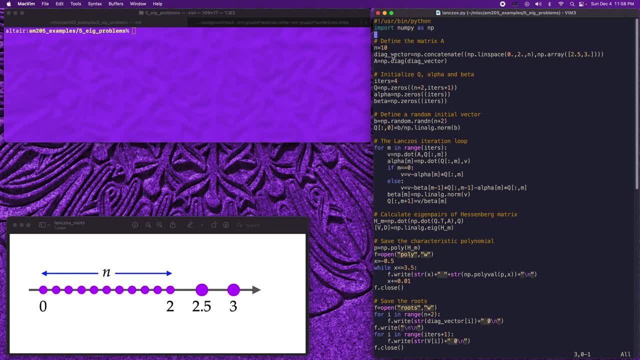 test case. So in the code we first define dieg vector to be the set of eigenvalues, so we have the linearly spaced set, and then we also add in the isolated values at 2.5 and 3 and we then compute a diagonal matrix from the dieg vector so those eigenvalues will 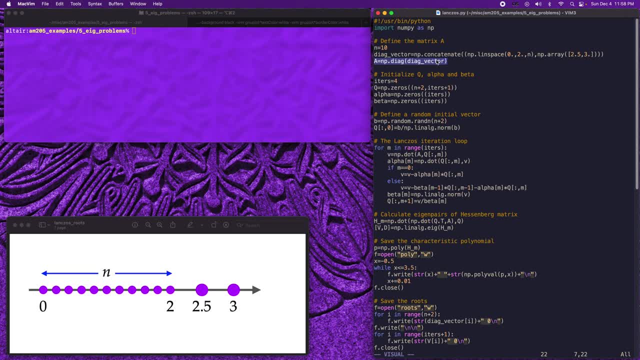 just be in the diagonal entries of this matrix. We'll then initialize the Q matrix that we'll use in the Lansosh algorithm, as well as the alpha and beta parameters that are used, and we'll then define a random initial vector, b, that's used to find the eigenvalues of the Lansosh algorithm. 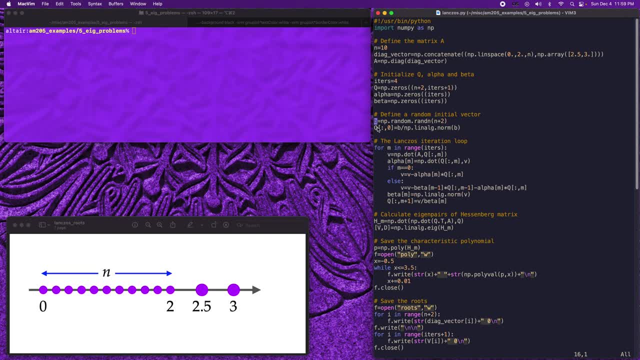 Here this inicial vector of b is set to 0 and the threshold is set to where the alpha value appears on the animation in Lansosh to generate the sequence of Krylov subspaces. and then the first column in our matrix Q will just be given by a normalized copy of b. 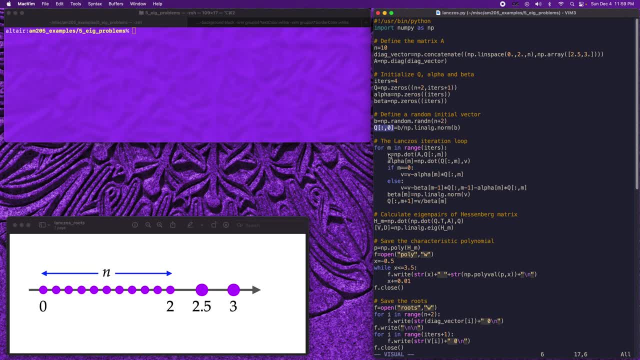 We'll then perform the Lansosh iteration and we'll perform the steps where we first compute the product A times Q and we then compute alpha at this stage and we then enter losers, adjust v using alpha and beta and we then compute the, the new beta, and at the end we get a new. 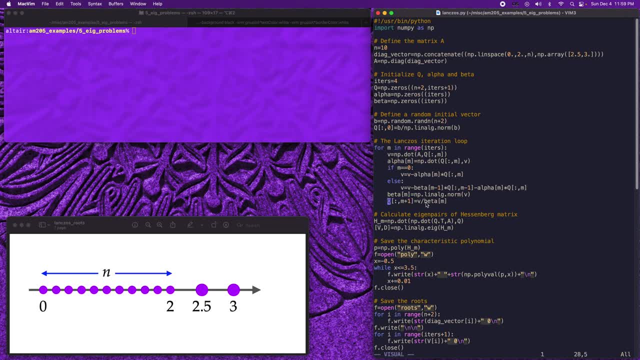 column of q by normalizing that vector v. Once we have this, then we can compute the associated Heisenberg matrix by calculating q, transpose times a times q, and we'll then compute the eigenvalues of this Heisenberg matrix. and here we're just going to make use of NumPy's. 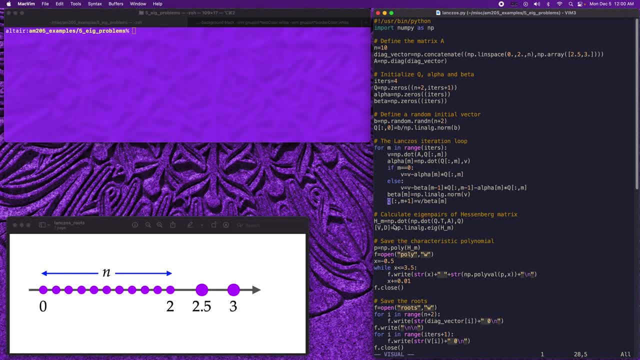 eig routine. however, we could use a custom algorithm, such as some of the approaches considered earlier in this unit. We'll then save the characteristic polynomial of the Heisenberg matrix using the NumPy dot poly routine and we'll sample this polynomial over the range from: 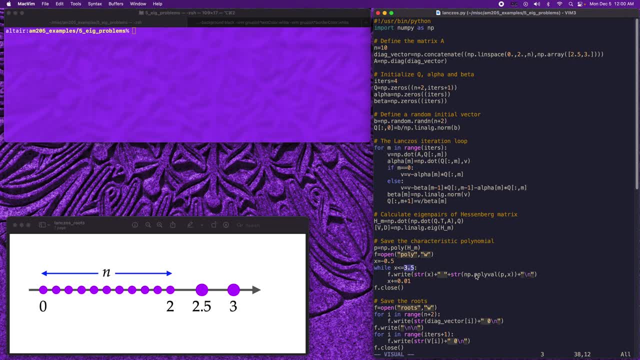 minus 0.5 to 3.5. using the polyval function, We'll also save the roots of the polynomial into a file called roots, and we'll first add the true eigenvalues of our matrix that are stored within die vector, and we'll then put in a few new lines and store the eigenvalues of. 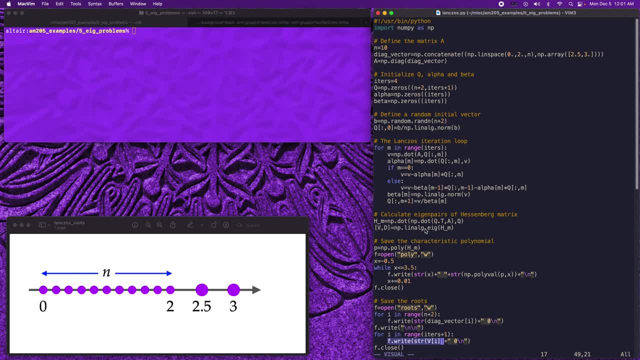 the Heisenberg matrix, that would correspond to the roots of the characteristic polynomial. So in this case, here we have 12 eigenvalues and we're going to perform four iterations of the Lansos algorithm, and so in this case, then, we're only going to get a small subset of. 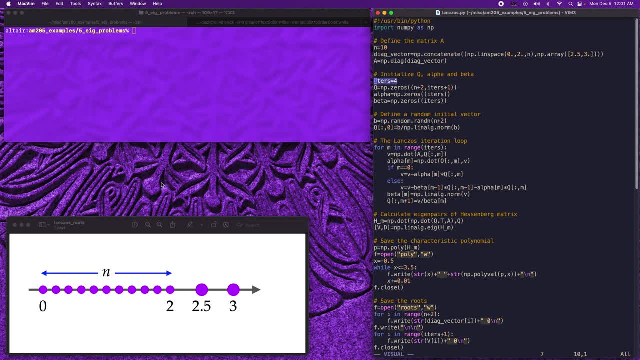 Ritz values that approximate the eigenvalues of the, the full matrix. So let me now go ahead and run this program and we'll now look at GNUplot to look at the output of the program. So first i'm going to plot the roots of the characteristic polynomial of the original matrix. 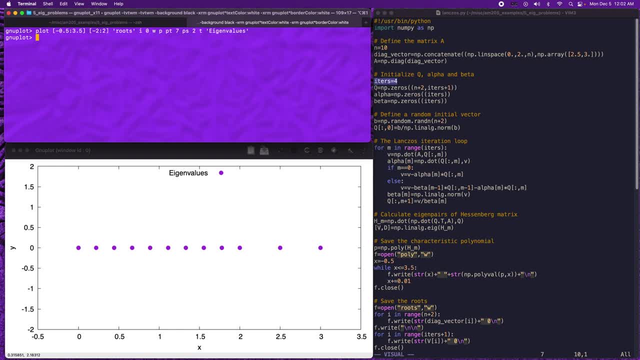 which could correspond to the eigenvalue of the original matrix eigenvalues. And I'm now going to add the characteristic polynomial of the Heisenberg matrix here that's stored in this file called poly. And so we see in this case that this characteristic polynomial has one root that very closely aligns with the eigenvalue at 3.. And this: 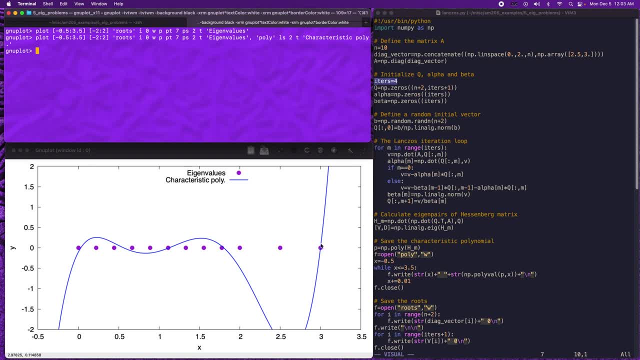 is as we would expect, since we expect it to catch these extreme values very well. And then this polynomial also has four roots that are distributed among the range from 0 to 2.. And currently we see that the value of 2.5 is actually far away from a root of the characteristic polynomial. So 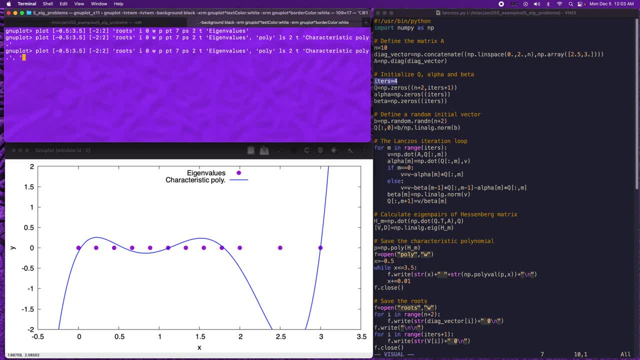 we could also add the specific roots of the characteristic polynomial that I also stored in the roots file, And these will correspond to the writs values. So let's now look at how we can get better accuracy for this test case. So let's first 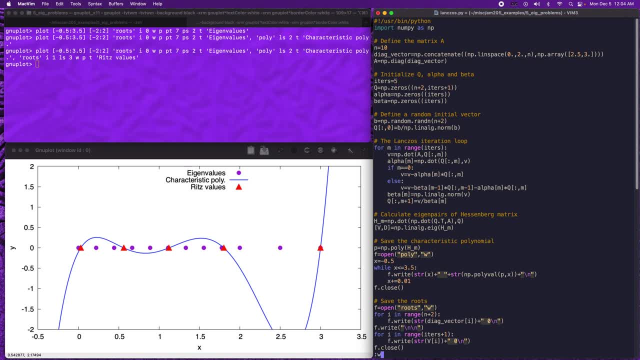 increase the iterations to five And we'll run the program again. And in this case now we see that two of the writs values get both the isolated eigenvalues of 2.5 and three quite accurately And we still have four writs values that are distributed among the range from 0 to 2.5 and 3 quite accurately. 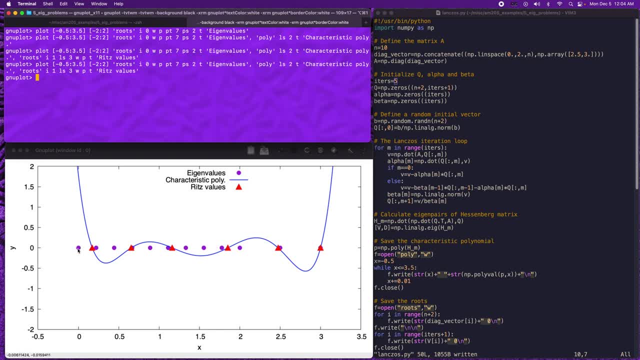 four Ritz values that are distributed over the range from 0 to 2.. So let's now increase the number of iterations further, and if we increase this to 11, then we should capture the complete spectrum of the eigenvalues of our test matrix, And so in this case then we can now see that we capture all of the 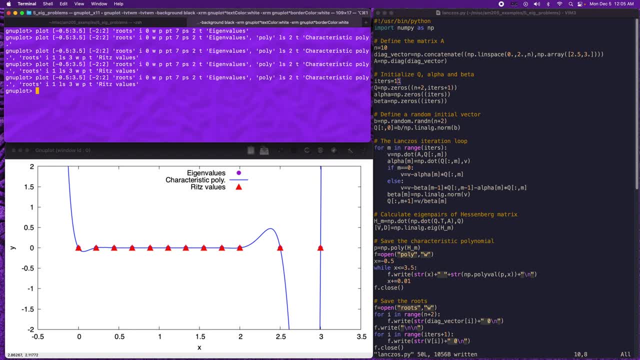 eigenvalues of our matrix accurately. So suppose now that we increase the n, the number of eigenvalues in that spread from 0 to 2, and we'll increase this to 11.. So let's now increase the number of eigenvalues in that spread from 0 to 2 and we'll increase this to 11.. So let's now 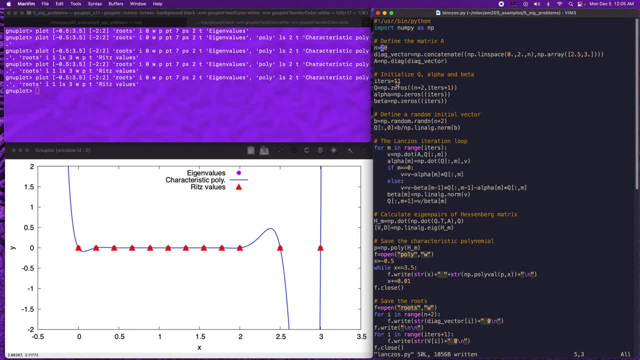 increase the number of eigenvalues in that spread from 0 to 20 and we'll keep 11 iterations of the Lansos algorithm. So now again, we're not going to be able to recover the precise eigen spectrum, but we should be able to do fairly well. 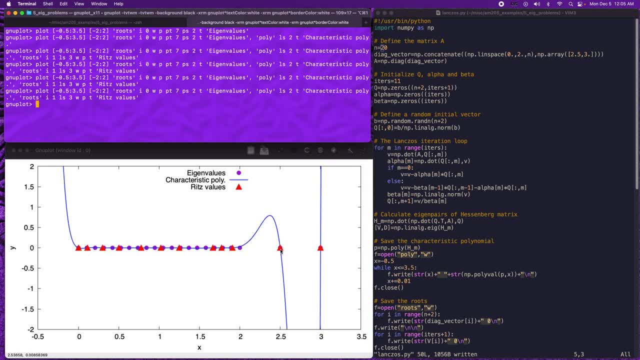 And so we see that we capture those two isolated eigenvalues well in this case, and then we have some spread of Ritz values over this range from 0 to 2.. So finally, let's look at what happens if we increase the iterations of the Lansos.